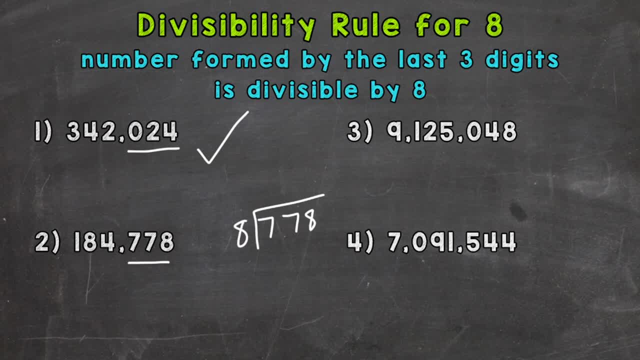 quick division problem. So we can't do out of the 7, so we need to go to the 77.. 77 divided by 8. That is going to give us 9 whole 8s. It gets us to 72. 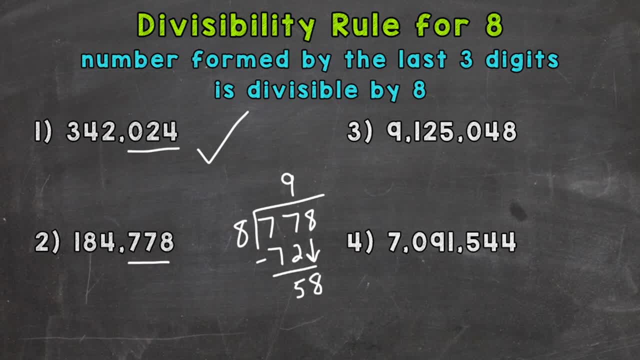 Subtract, we get 5.. Bring down the 7., 8., So 58. How many whole groups of 8 out of 58?? Well, 7.. That gets us to 56. And we get a remainder of 2.. 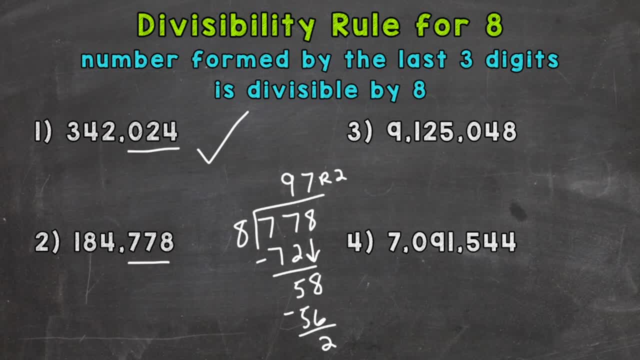 So 97 remainder 2.. 778 is not divisible by 8.. Therefore, our original number of 184,778 is not divisible by 8 either. So on to number 3, where we have 9,000,000.. 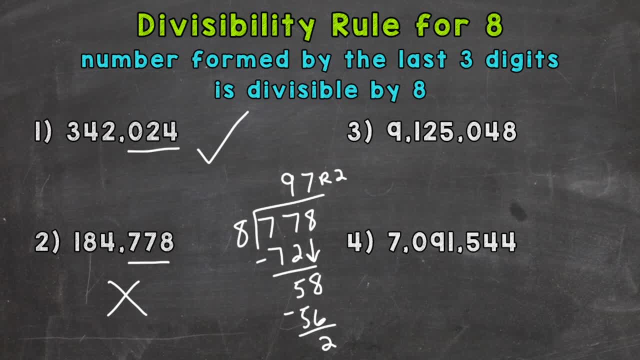 125,048.. So our last three digits gives us a 48 there, And 48 is divisible by 8.. 48 divided by 8 equals 6, without a remainder. Since those last three digits are divisible by 8, 9,125,048 is divisible by 8 as well. 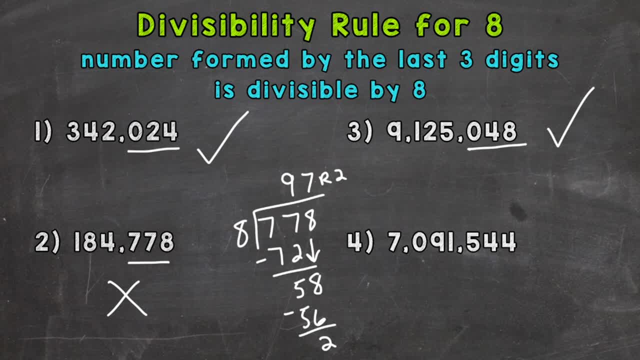 Now, lastly, number 4.. We have 7,091,548.. 7,091,548.. 544.. So our last three digits here: 544.. I'm not sure, off the top of my head. so let's do a quick division problem. 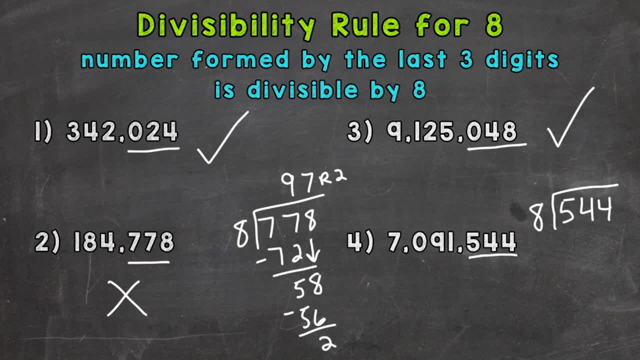 Off to the side here, And we'll start with 54 divided by 8.. So how many whole groups of 8 out of 54?? Well, 6.. That's going to get us to 48.. We'll subtract And we get 6.. 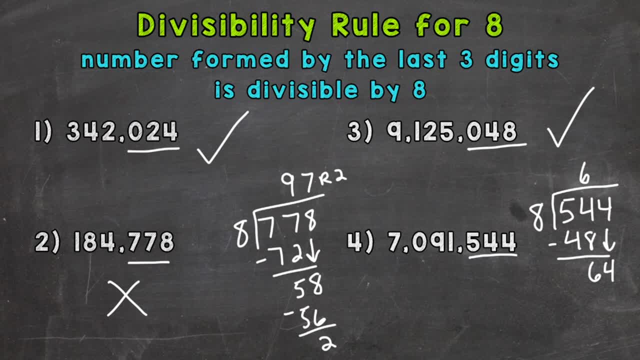 Bring down our 4 here And 64. And 8 are compatible. So 64 divided by 8 gives us an 8.. 8 times 8, 64. And that shows that we do not have a remainder. So 544 is divisible by 8.. 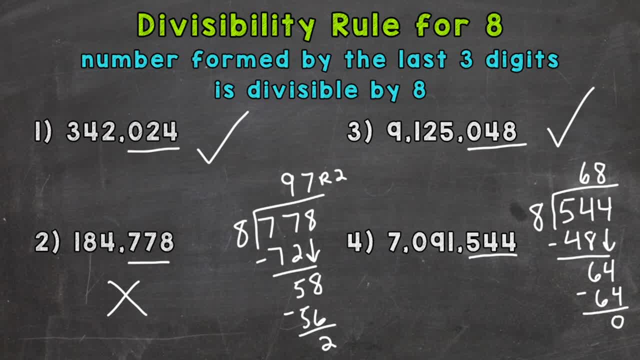 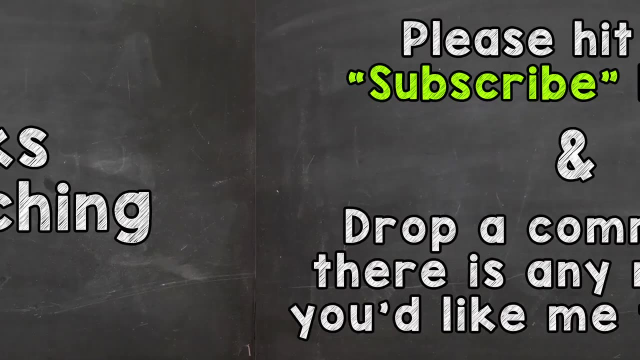 Therefore, our original number of 7,091,544 is divisible by 8 as well. So there you have it. There's the divisibility rule. We now have an integral for 8.. I hope that helped. Thanks so much for watching.